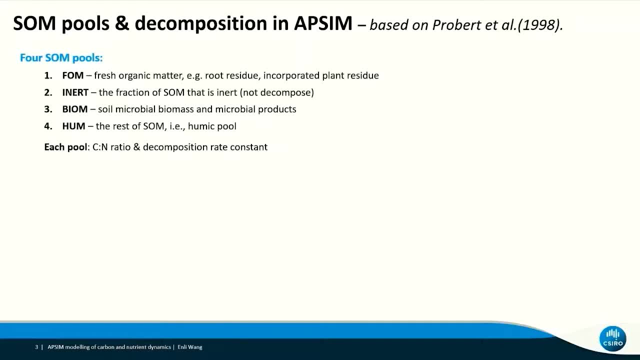 The second one is the inert pool, referring to the fraction of soil organic matter that is inert and does not decompose. The third one is the balm pool for soil, microbial biomass and microbial products. The last one is the HUM pool, that is, the humic pool containing the rest of soil organic matter. 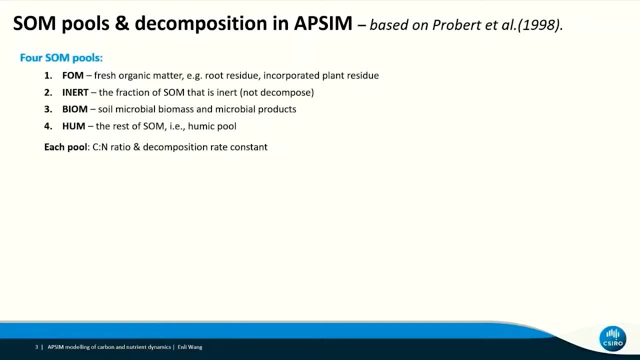 Each of the pools has its own C2N ratio and a potential decomposition rate. constant Decomposition is simulated in Epsom as a first-order decay process. Decomposition of soil organic matter is a first-order decay process. Decomposition of soil organic matter is a first-order decay process. 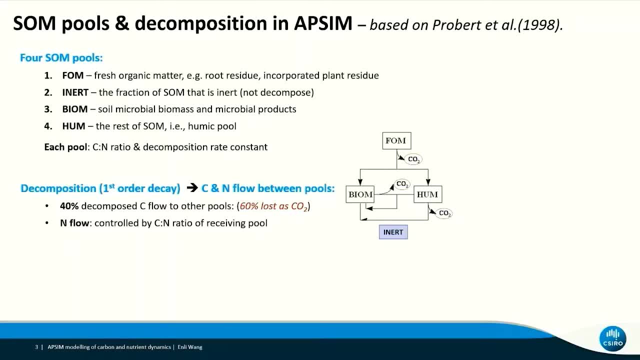 When soil organic matter decomposes, 60% of decomposed carbon will be lost to the atmosphere as CO2.. When soil organic matter decomposes, 60% of decomposed carbon will be lost to the atmosphere as CO2., While 40% will be transferred to other pools. 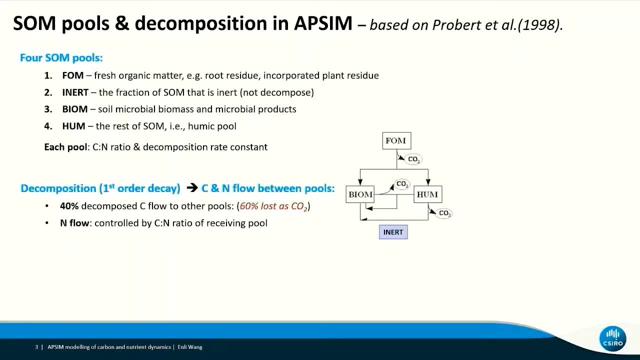 The nitrogen flow between pools is controlled by the C2N ratio of the receiving pool. The decomposition process also leads to mineralization. also leads to mineralization or immobilization of soil nutrients such as nitrogen. The released nitrogen from decomposition in the form of NH4 can. 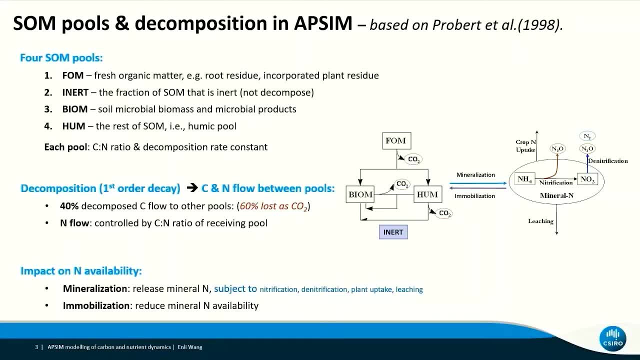 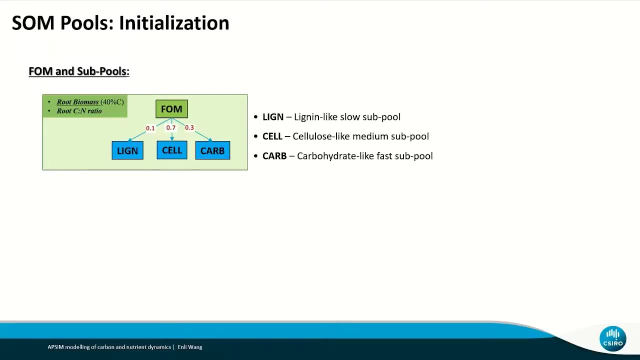 further go through the processes of nitrification and denitrification and is made available for crop uptake and leaching. All the SOM plots need to be initialized before running a simulation. The initial carbon and nitrogen amount of FOM is normally estimated using root biomass from previous season and root 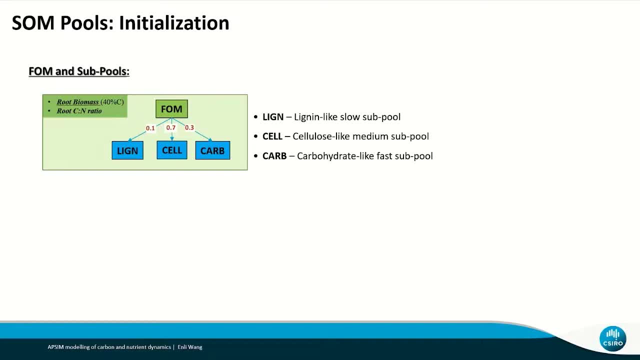 C2N ratio. FOM in Epsom is further separated into three sub pools, That's a lignin-like, a cellulose-like and a carbohydrate-like sub pool with increasingly fast decomposition rate. The initial sizes of the ENET, BAUM and HUM pools are: 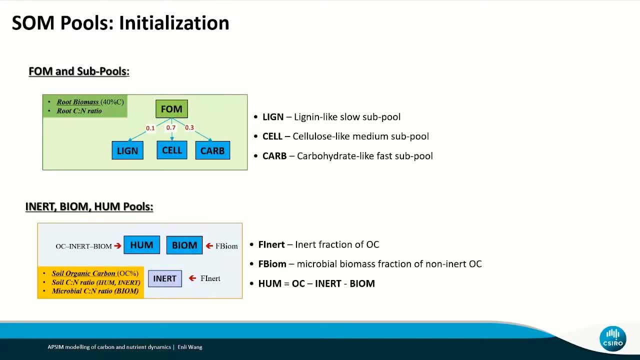 estimated using the soil organic carbon percentage, soil C2N ratio for HUM and ENET pools and soil microbial C2N ratio for the BAUM pool. Firstly, for the ENET pool, the carbon content is calculated using F-ENET, which is the ENET fraction of organic carbon For the BAUM pool. 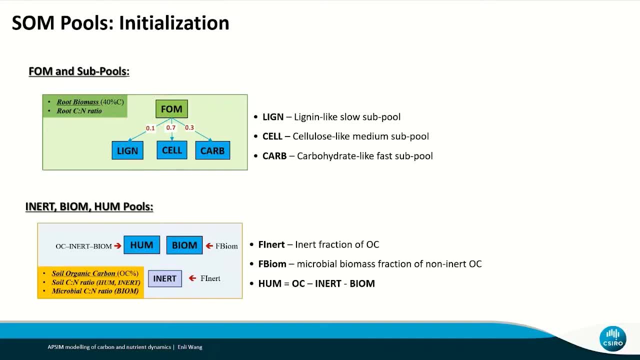 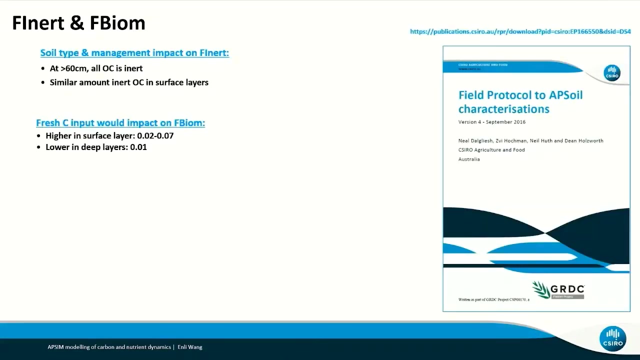 its carbon content is estimated using the F-BAUM, which is the microbial biomass fraction of the non-ENET carbon. After the ENET and the BAUM pools are initialized, the remaining carbon is put into HUM. For F-ENET and F-BAUM, there is an online document available, prepared by Neil. 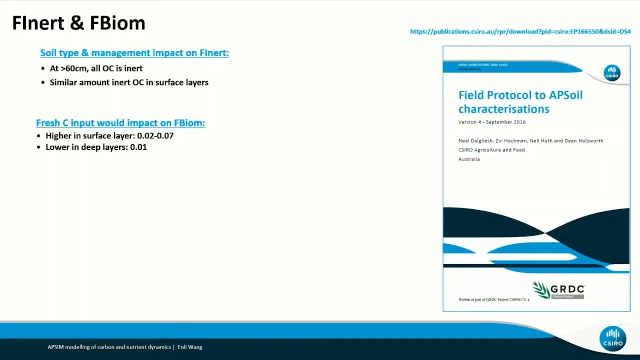 Deglish and other CSIRO colleagues. A section in this document describes how to estimate F-ENET and F-BAUM. Basically, F-ENET can be affected by soil type and management. Normally we can assume that all carbon below 60 cm in soil is ENET and the surface layers have a C2N ratio. 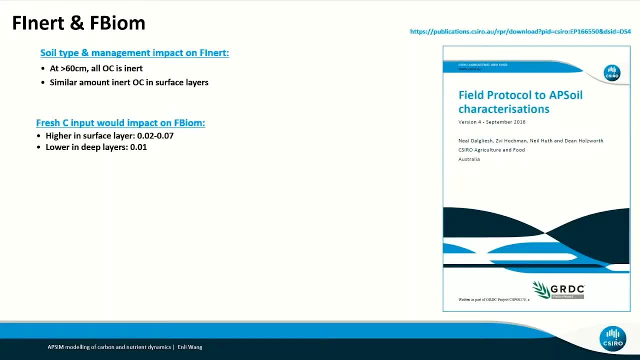 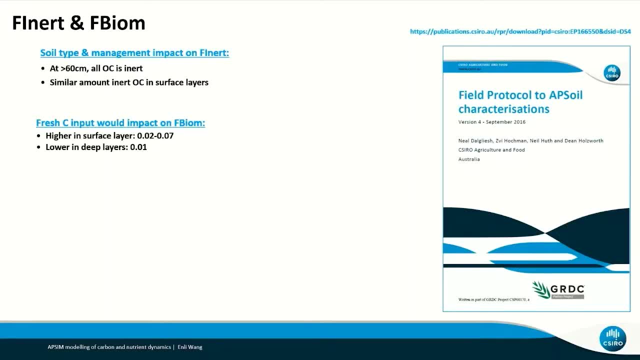 Normally we can assume that all carbon below 60 cm in soil is ENET and the surface layers have a C2N ratio. This enables estimation of Fe with soil carbon and measurements in different soil layers For F-Balm. it is affected by fresh carbon input. 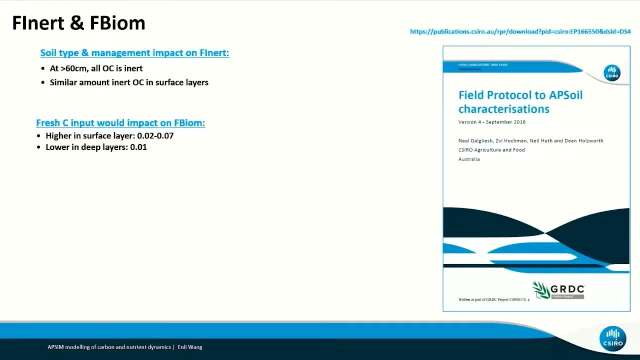 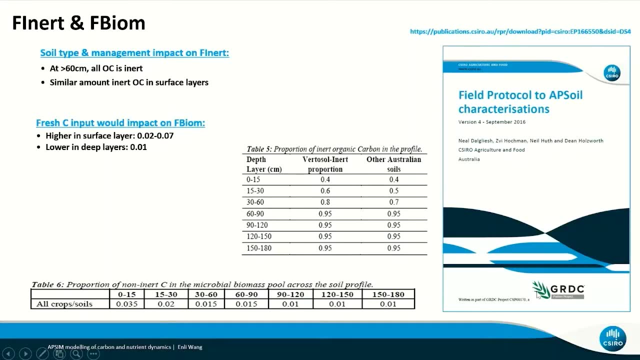 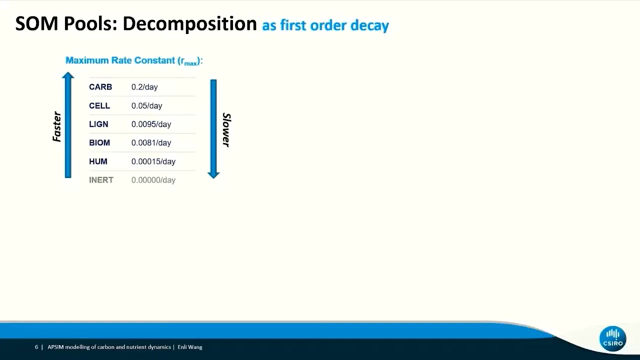 So it is higher in surface layers and lower in deeper soil layers. The two tables show some indicative values for Fe and F-Balm for typical soils in Australia. They are from the document on the right. Once the SOM pools are established, EPSIM simulates their decomposition as first-order. 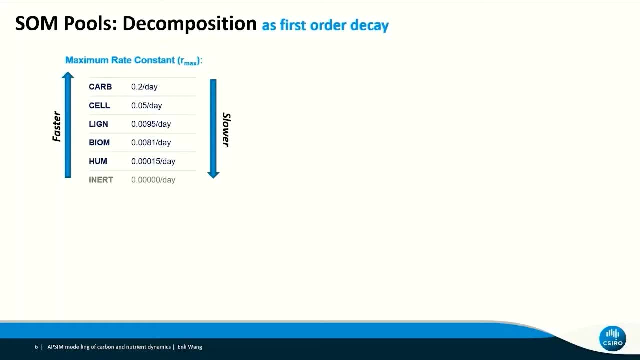 decay using rate constants. Each SOM pool has a maximum rate constant as listed in this table, with the quickest pool on the top and slowest pool at bottom. The inert pool was auto-pooled In the simulation. the actual rate constant is simulated as the maximum one, modified by 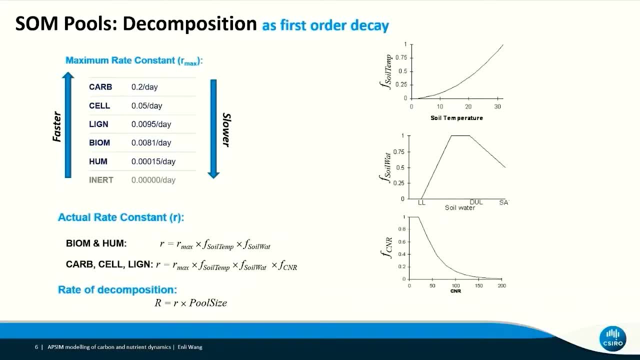 a temperature and soil water factor for Balm and Hume pools and an additional soil CN ratio factor for the three FOM subpools. The actual rate of decomposition is the rate constant multiplied with the size of each pool. The graphs on the right show the responses of decomposition rate to soil temperature. 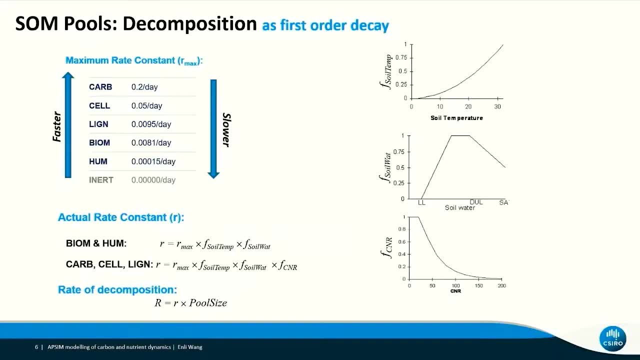 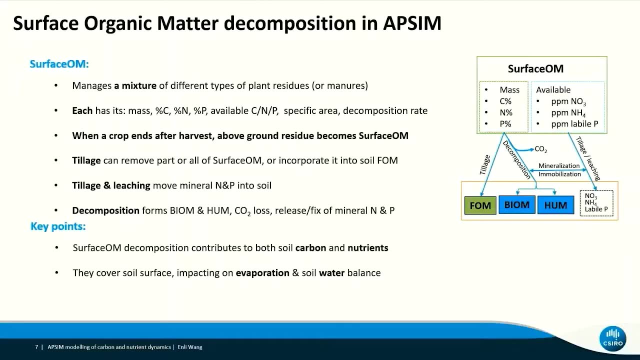 on the top, soil water in the middle and soil CN ratio at the bottom. A further point of attention is the decomposition of the surface organic matter in EPSIM. This is handled by the surface OM component. The surface OM can manage a mixture of different types of plant residues or manures. 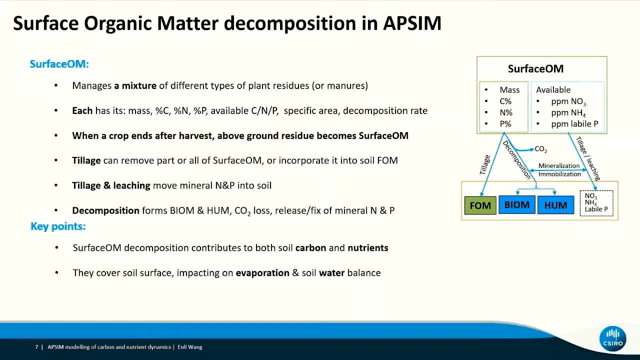 Each can have its own mass nutrient contents in organic and mineral forms, specific area and decomposition rate: constant. When a crop is ended after harvest, its above-ground residue becomes surface organic matter and the root residue becomes fresh organic matter in the soil. 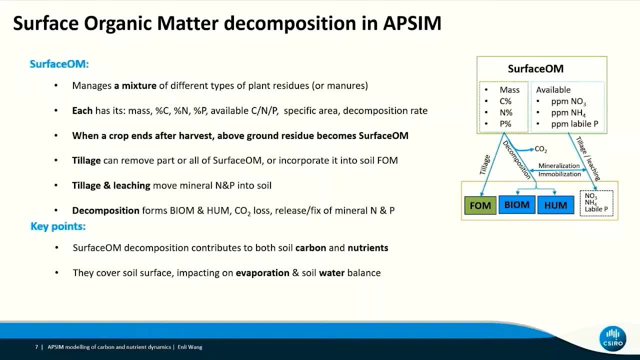 Different tillage options can be used to remove a fraction of surface organic matter or incorporate it into soil to become FOM. Decomposition of surface organic matter forms new Balm and new Hume, releases CO2 and also releases or fixes mineral nutrients such as nitrogen and phosphorus. 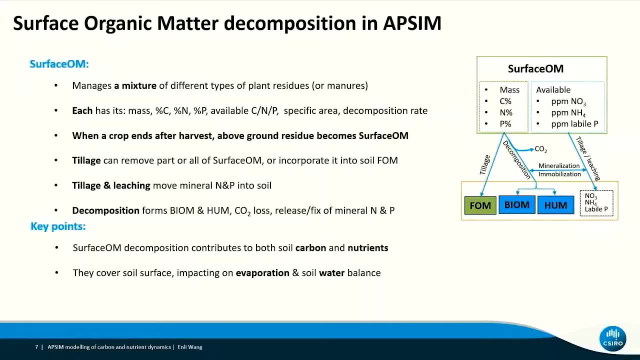 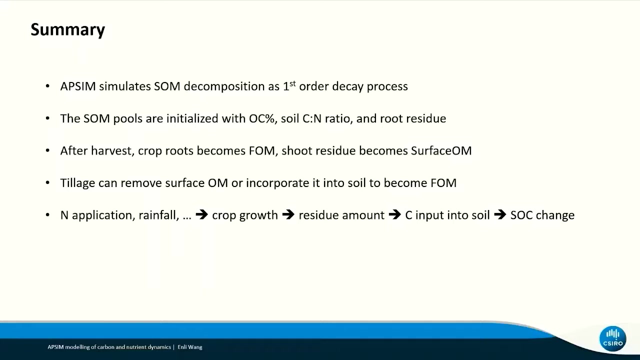 I don't want to go into details, But two key points to remember here. firstly, surface OM impacts on both soil carbon and nitrogen and secondly, surface organic matter covers soil surface can impact on evaporation and soil water balance. To summarize, EPSIM simulates soil organic matter decomposition as